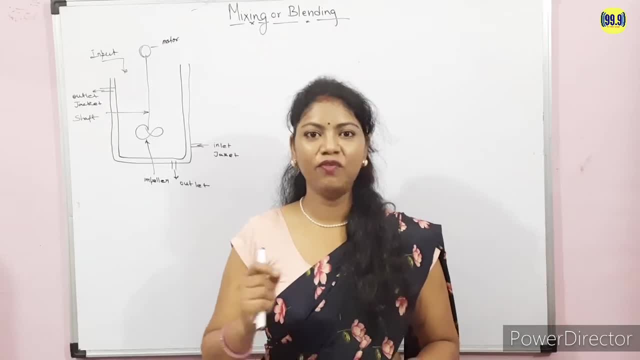 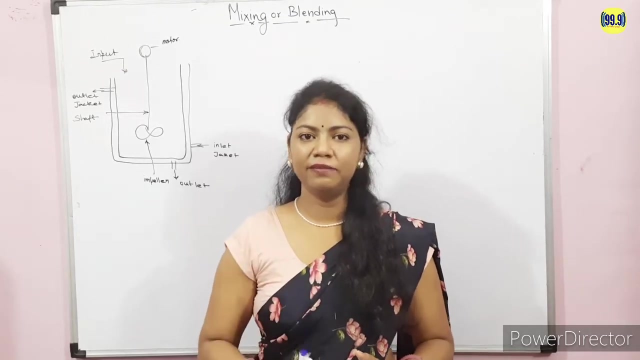 with the lecture. So basically, the mixing is the process of putting together two or two more than two dissimilar particle in the same system. So mixing are different type, like liquid liquid, mixing gas, liquid solid, liquid liquid solid. So these are the types of the different types of 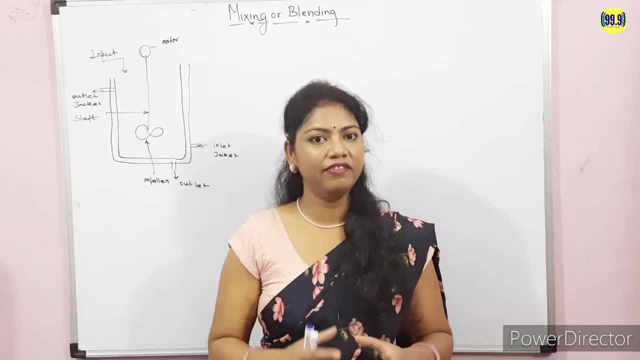 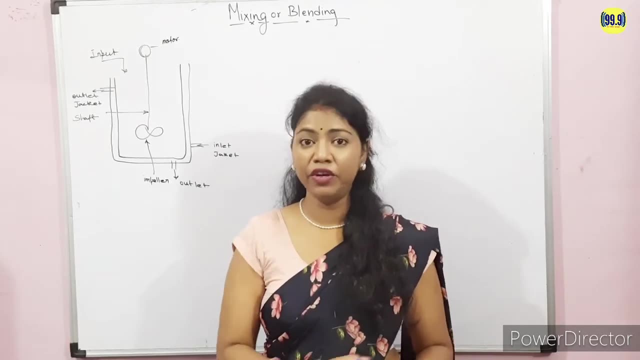 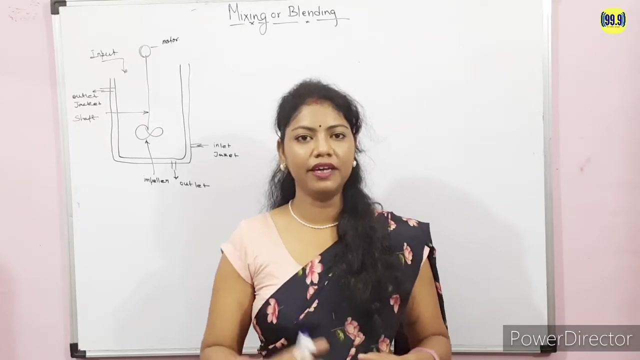 liquid mixing. okay, So basically, if we talk about the liquid liquid mixing, so basically it is a simple type of mixing and it is involves the formation of homogeneous system. If we talk about the gas gas lake mixing, it will be a seldom difficult, but you can, we can do it okay. 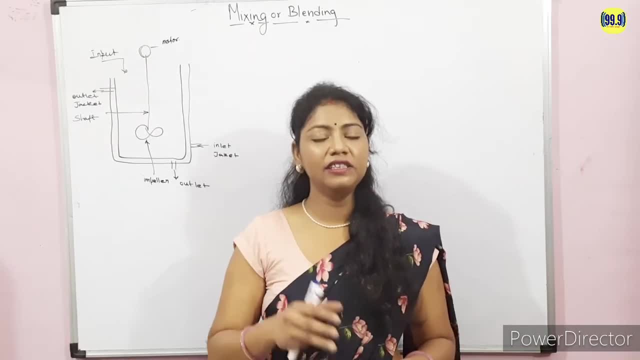 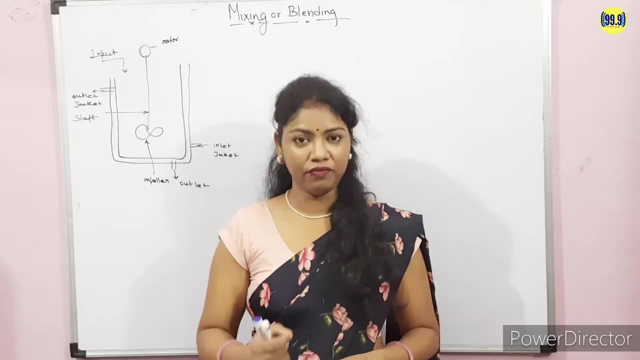 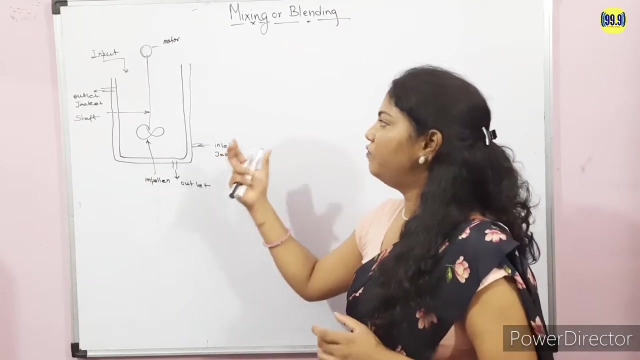 And the third one is the solid liquid mixing. it is a basically a little bit process and it involves the application of the shear forces. okay, so now we discuss the basically the basic diagram or schematic diagram of the vessel which which is used for the mixing. so this is the stainless steel vessels and it is 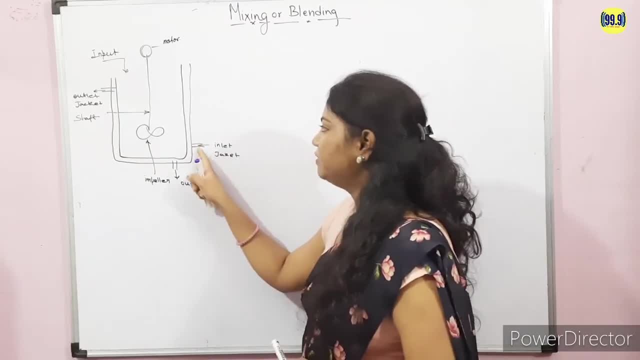 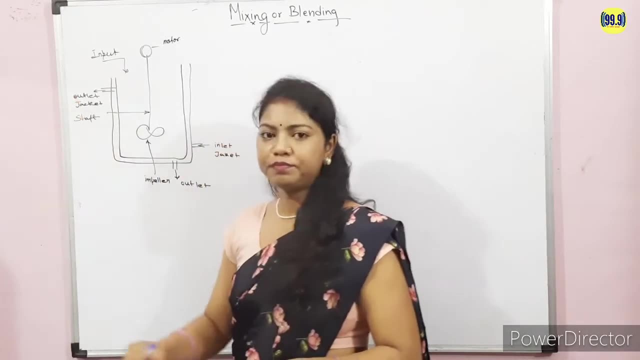 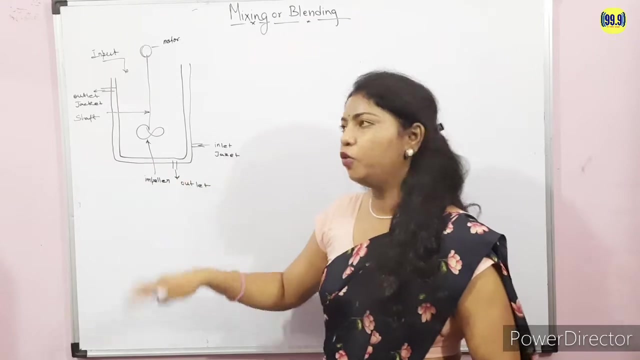 covered by the jacket. so this is the inlet fluid. from here we inserted the inlet fluid for this jacket and from here we get out the outlet of the fluid. from the jacket we inserted the input from here and from here we got the output. so main thing which is used for mixing, that is impeller which is used. 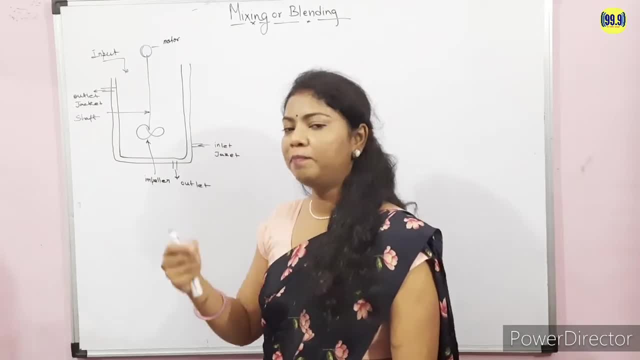 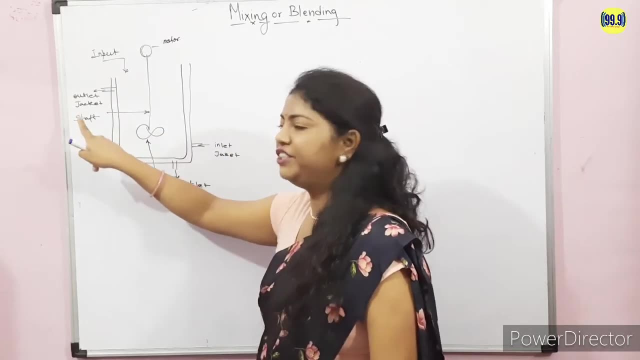 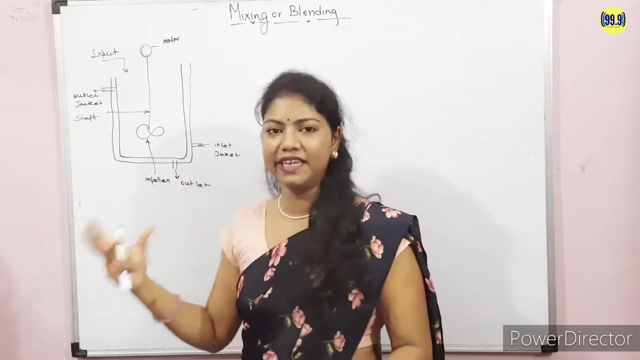 for mixing the material or particles with the, and it is mounted on with the help of shaft and shaft is drive by the motors. so this is the all about the mixing vessels, and it is made up of these stainless steel. so if we talk about the Flex B question and genesis, Round table 18. 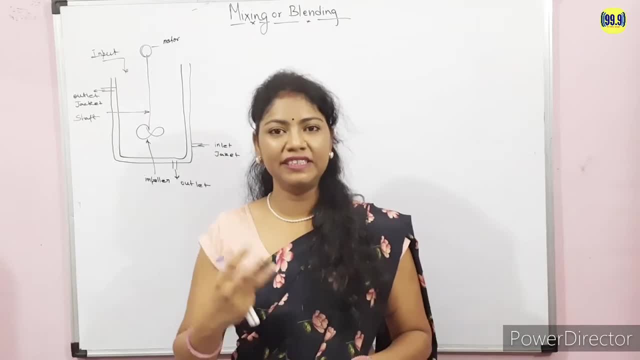 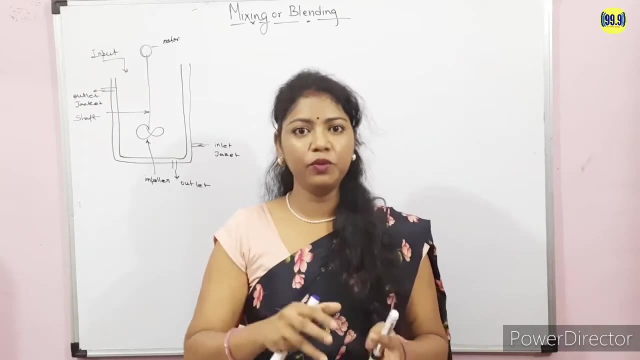 橋 들어가. Ihre Exodus in our video siet B of Mixing Day seriesası, the construction of this mixing vessel. it is the ratio of the 2 is to 1, that is, the tank dia to the tank height. it is the ratio of the tank dia or tank height is is the 2 is to 3. 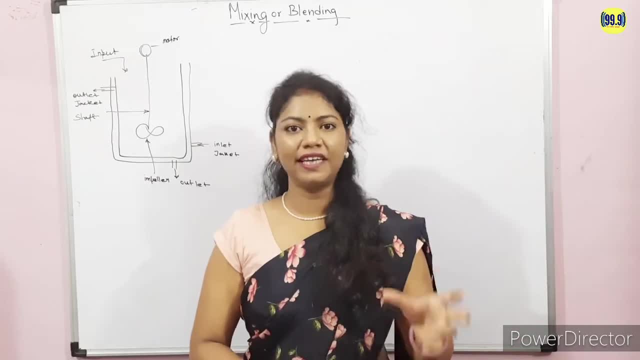 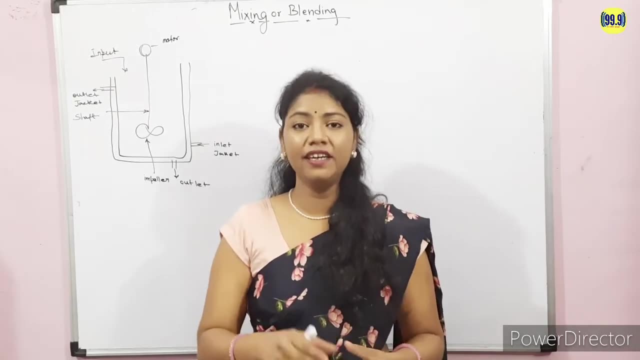 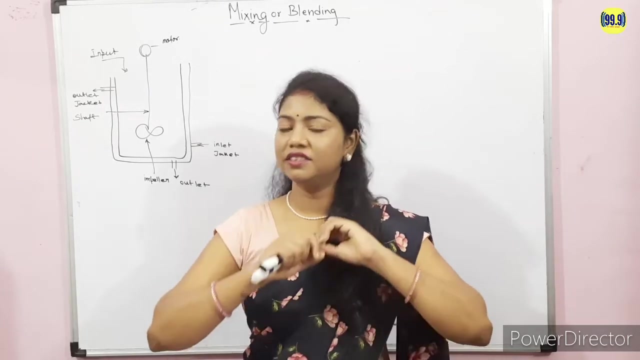 so basically, we also known the mixing process as a blending process. so in scientific language, in the scientific language, mixing is the process of mixing the weak liquid with weak steam with the concentrated steam. okay, so this is all about the mixing, about the mixing, and now we talk about 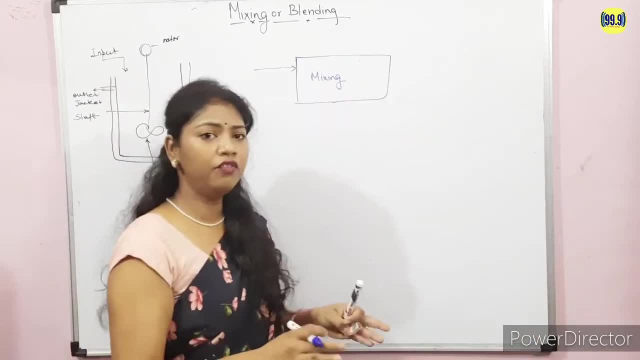 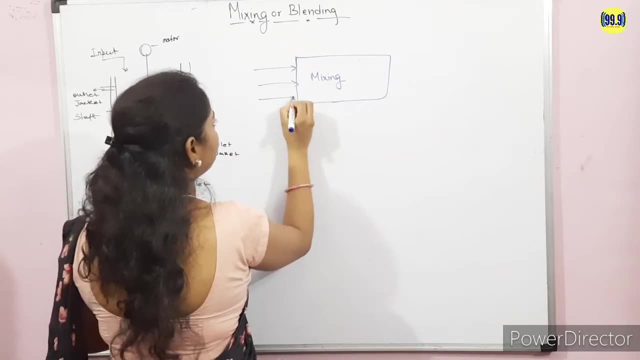 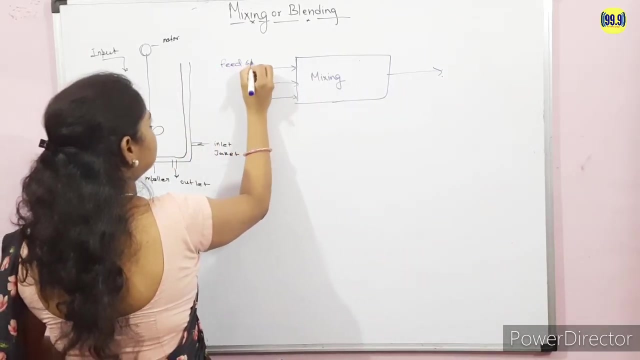 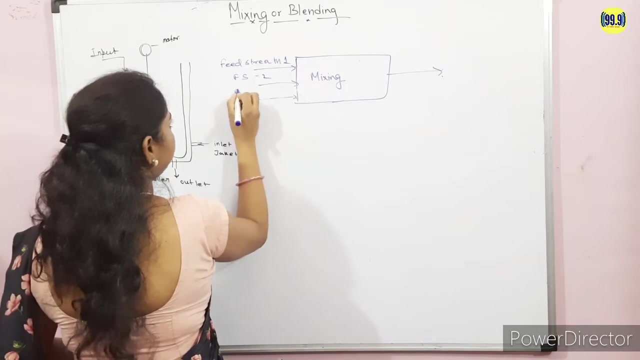 the material balance, about the of the mixing. now we do the material balance on the mixing. so we first draw the raw diagram or basic diagram, block diagram for the mixing tank. that is, from here we inserted the feed stream, stream 1, stream 1, feed stream 2 and feed stream 3, and from here we get the desired product. 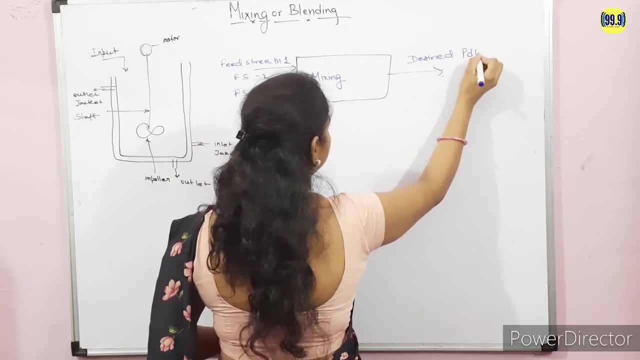 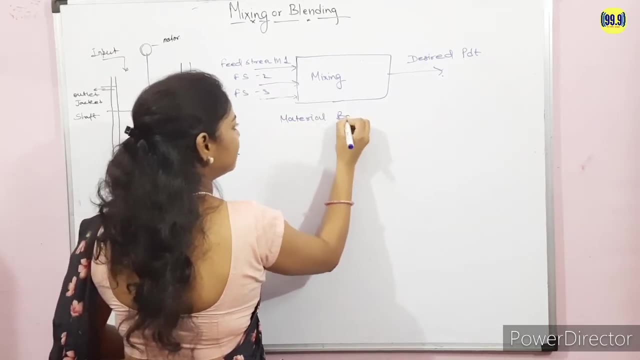 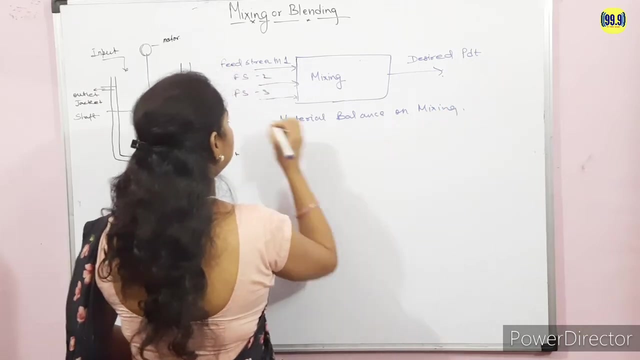 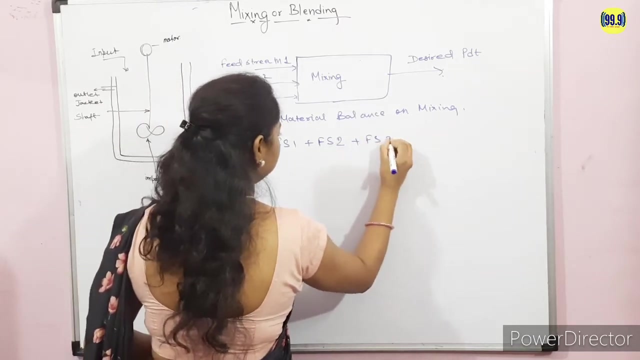 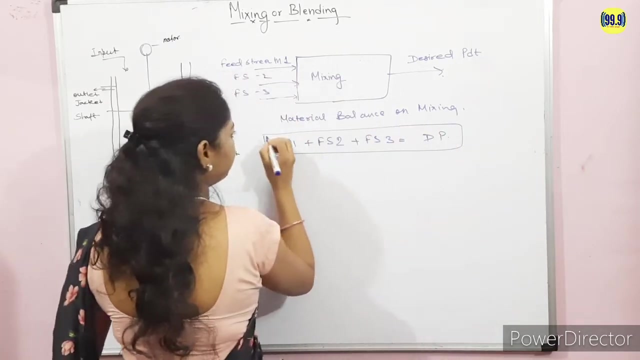 desired product. and if we want to write the material balance- material balance on mixing, mixing process- it will be. it will be: feed stream 1 plus feed stream 2 plus feed stream 3 is equal to desire product. so this is the raw, this is the material balance of the, this block diagram, mixing of the mixing process. so it is. 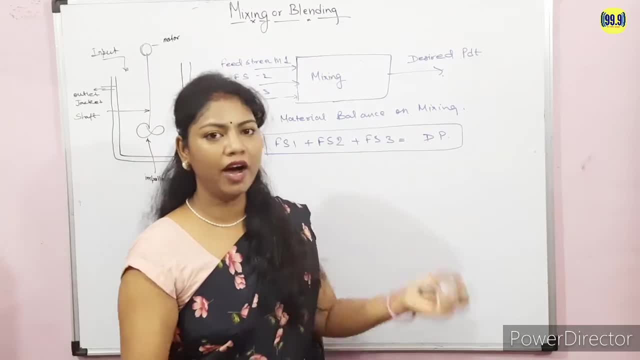 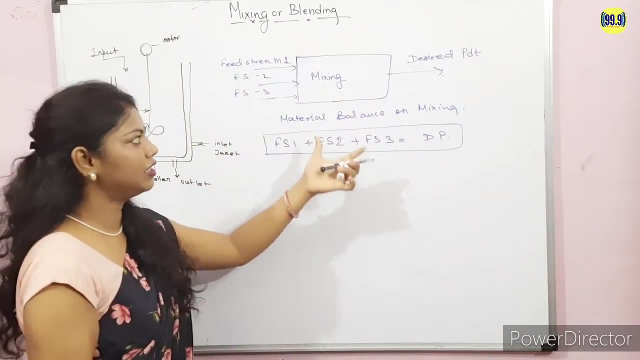 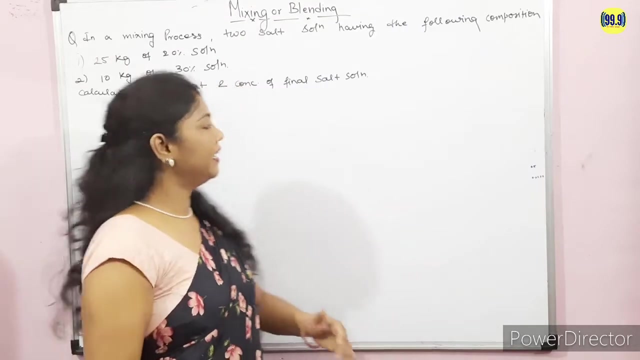 a, simply the input, all the input, is equal to output. so now we are going to discuss some numericals based upon the blending process and, as i said earlier, what is thelist of material balance based upon the blending process? and, as i said earlier, i already said that the mixing is all also known as the blending process. okay, so the question is: 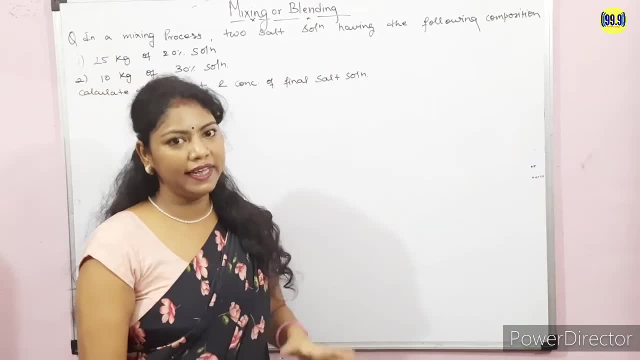 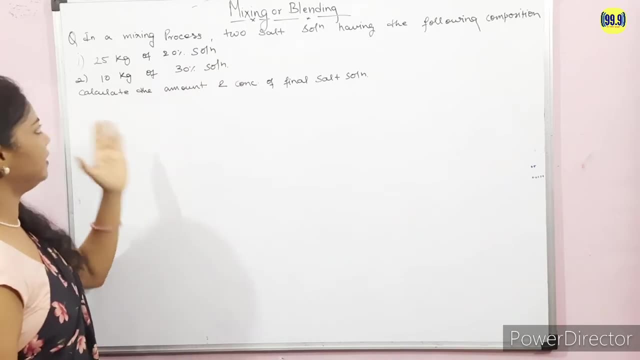 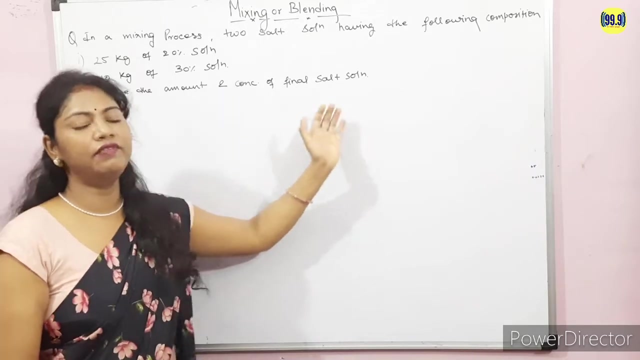 in a mixing process, two salt solution having the following composition: the first one is the 25 kg of the 20 percent solution and the second one is 10 kg of 30 percent solution. so we have to find out the amount and the concentration of the final salt solution. okay, so let's draw the mixing. 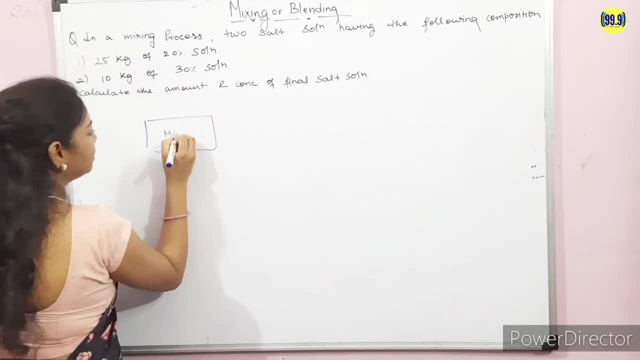 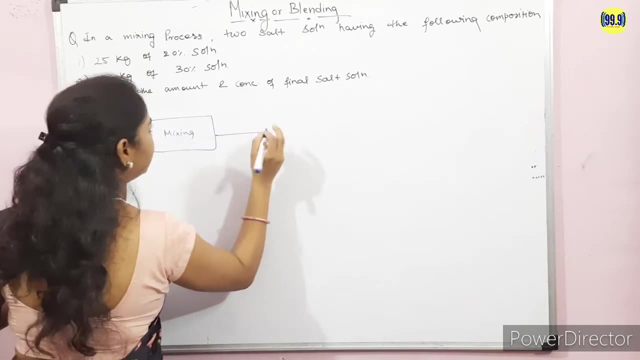 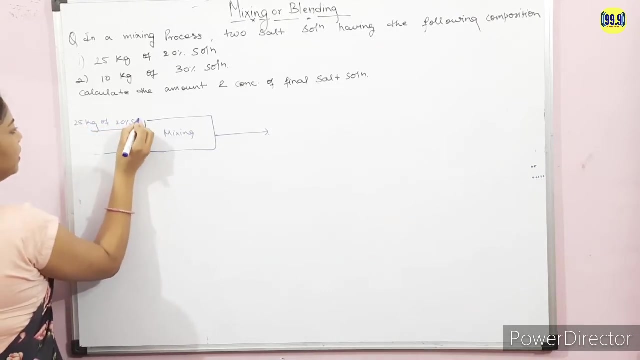 process block diagram. that is, it is a mixing process. the first stream which is coming into the mixer and the desired product is like that: first one is the 25 kg of 20 percent solution and the second one is the 10 kg of 30 percent solution. okay, so this is the all the given data. 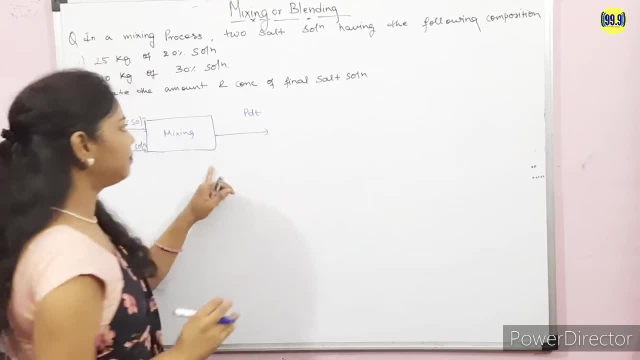 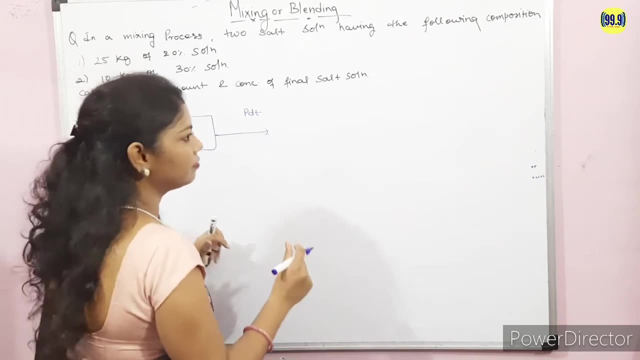 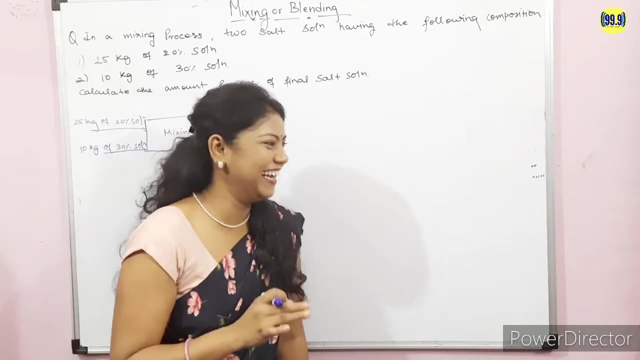 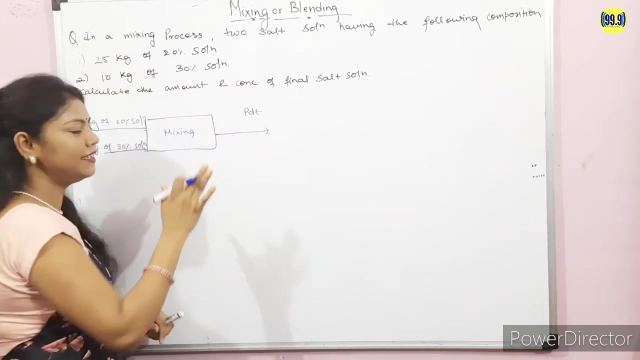 of the product. okay, so now we first apply the overall balance on the mixing process, then we apply the material balance on it. okay, basic. so basically first we have. so. so basically, we first apply the material balance- overall material balance- and then we apply the component balance, or then we apply the component balance on it. so first, 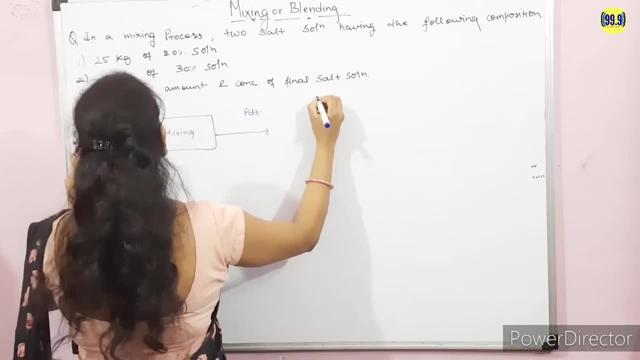 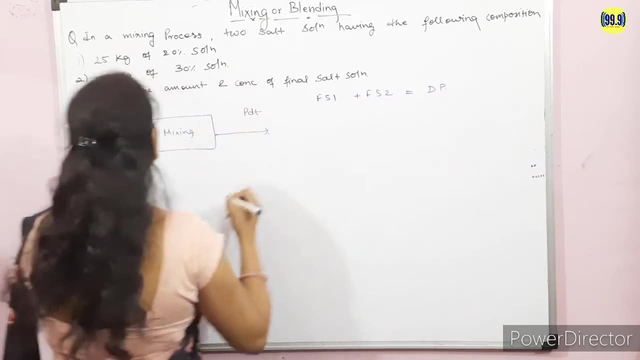 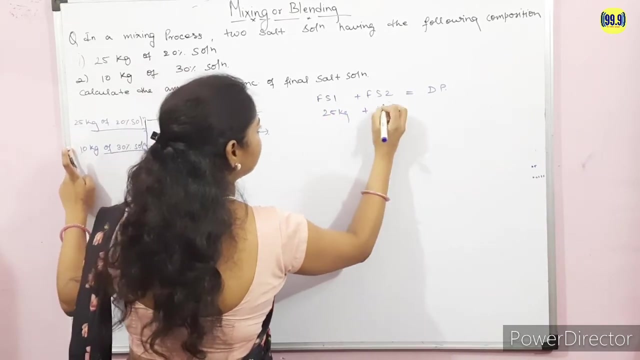 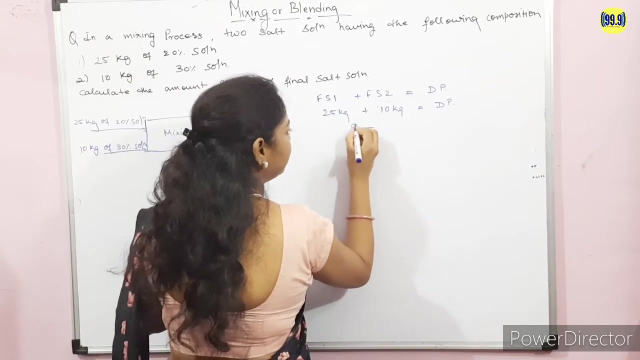 we input stream. all the material input stream is like feed stream 1 plus feed stream 2 is equal to desired product. so feed stream 1 is contained 25 kg plus 35 kg, 10 kg, 10 kg and the desired product which we get from here. that is total. that is. 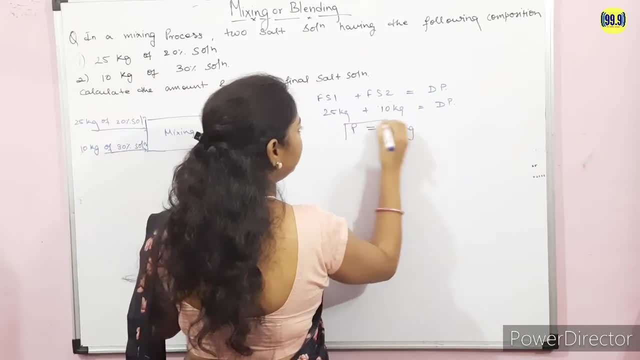 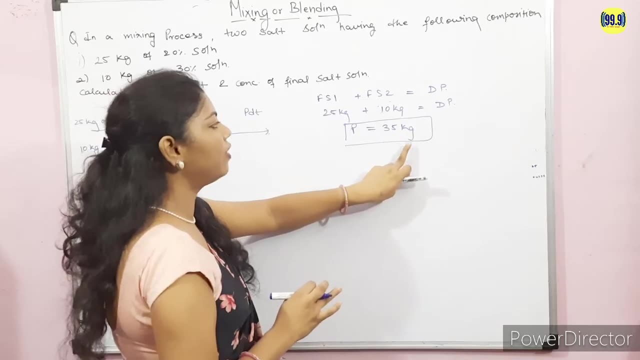 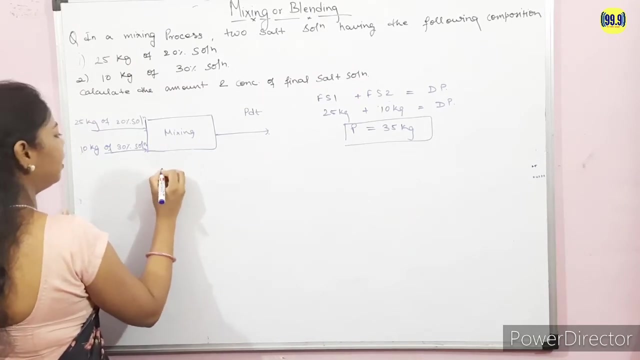 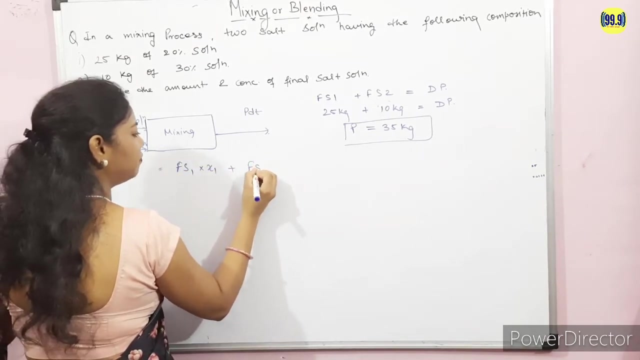 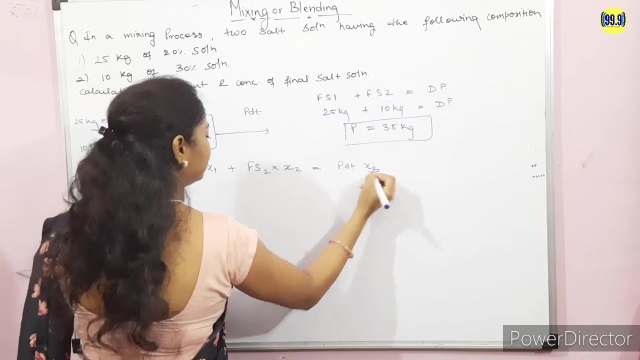 product is 35 kg. so we all. Now all the output, or the output of the salt solution is the amount of output of this salt solution is 35 kg. Now apply the composition balance, that is, feed stream 1 into X1 plus feed stream 2 into X2 is equal to product and X2- X3. 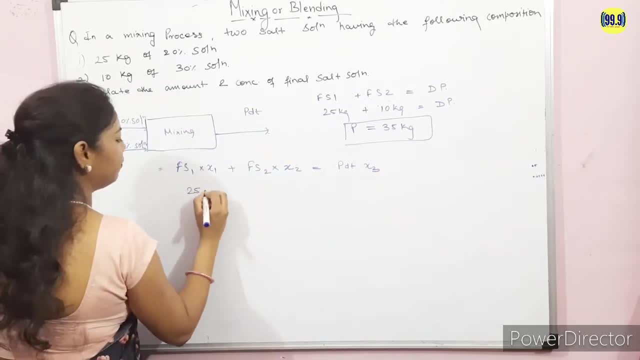 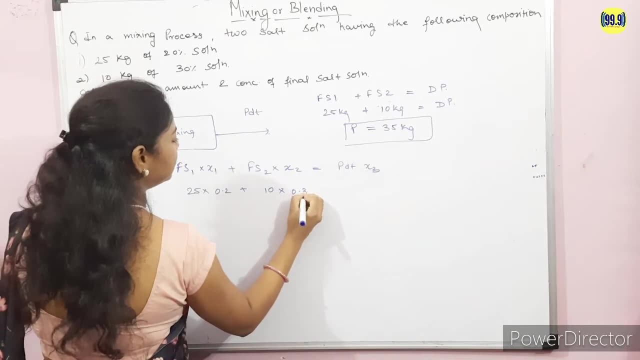 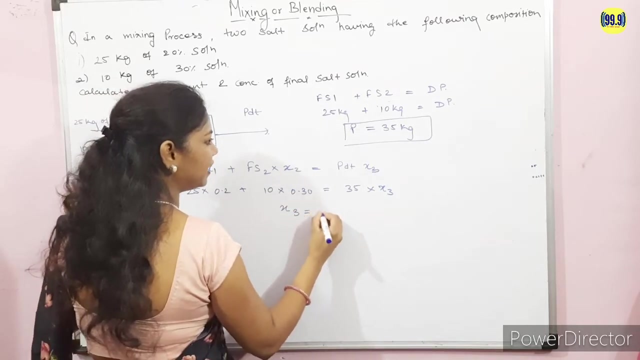 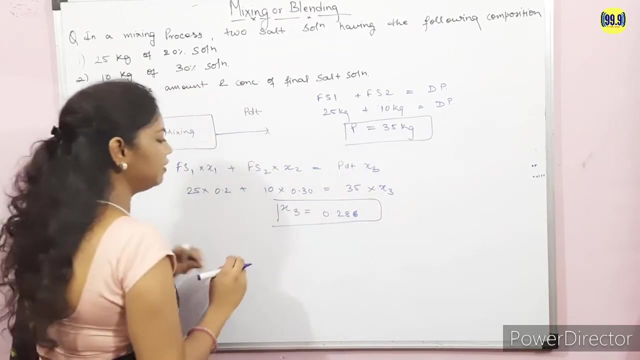 So we have applied here: 35 plus 25 plus 0.2 plus 10 into 0.30 is equal to 35 into X3 and from here we get the value of S3 is 0.286.. So this is the value of the X3 composition, which is the concentration of final solution. 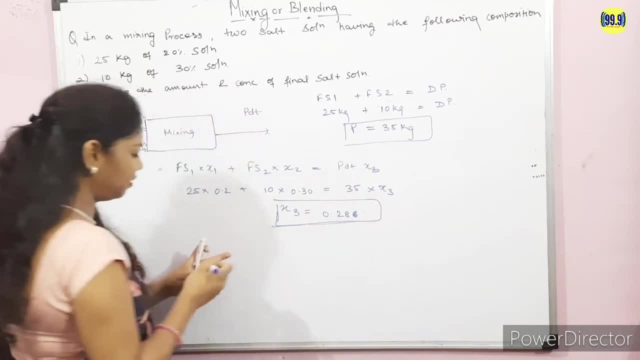 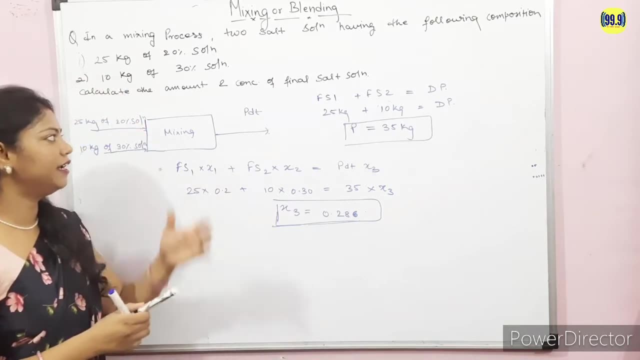 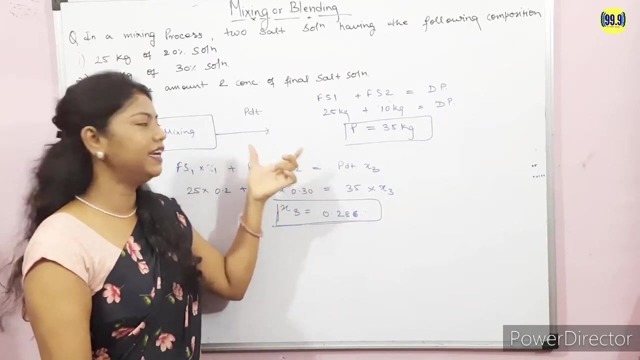 That is X3 0.286.. Okay, So the question is very simple, like that. You have to solve, You have to concern about the stream, The amount of input which is coming in the system and the amount of thing is out from the system. 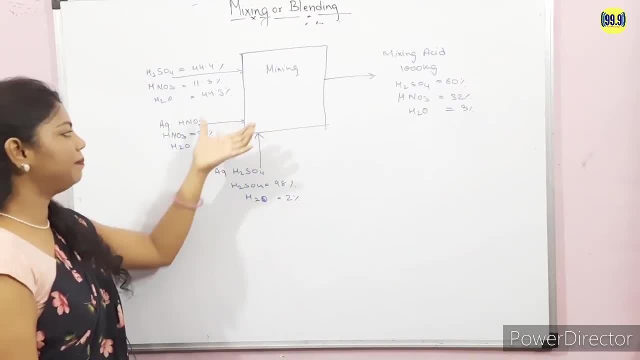 Okay So. second question is also based on mixing. We have three feed stream and one output. Okay, So the composition of feed stream I have noted down here, Okay, Okay, How much percentage of H2 SOF from the water goes into H2 and CO4??